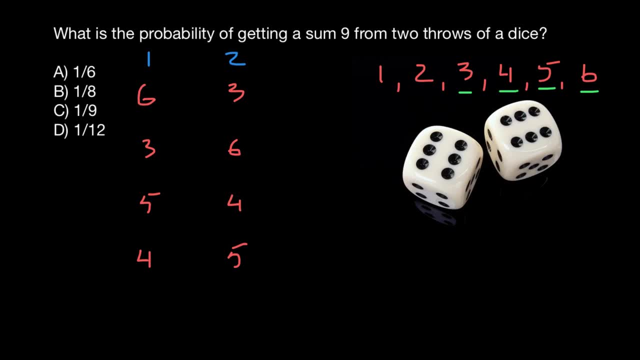 to find that, for example, we'll get six if we'll throw one down dice. and because dice has six surfaces, the probability that we'll get six would be one six. so one six that we are going to get six, and probability that with the second attempt, we are going to get three would be. 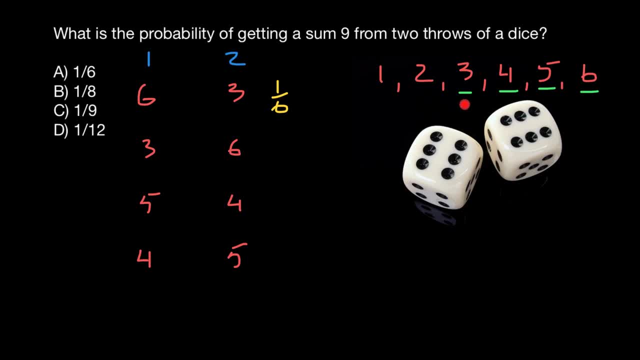 also one six. so we have a six variants and probability that this is going to be three would be one out of six. so probability that with the second attempt we'll throw dice and would be three, one six. so we have to multiply these two numbers in order to find. 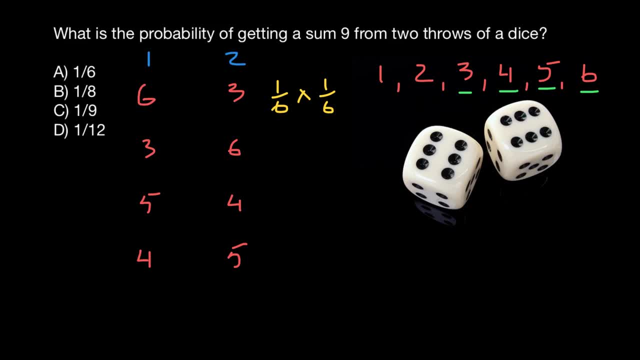 probability that in first attempt we are going to get six and in second attempt we are going to get three. so we have to multiply these two variants and we are going to get one over 36. this is going to be a probability of this combination and the same is true here. we are going to get probability one. 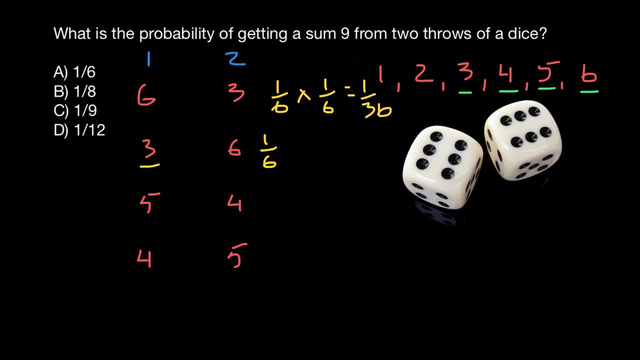 six, that we are going to get three in our first attempt and probability that we are going to get six in the second attempt also would be one six. so probability would be one over thirty six. one six here, one six here again, would give us one over thirty six. the same is true for 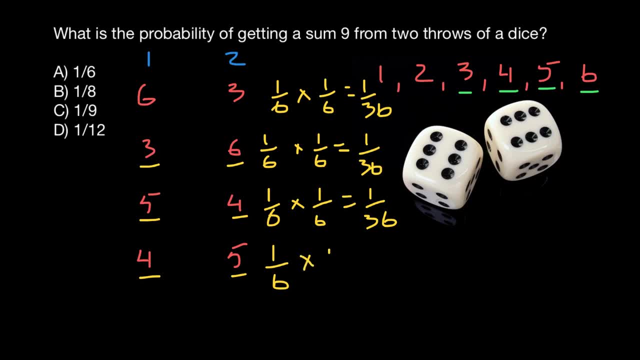 these two numbers, one six and one six, would give us one over thirty six. so all these four combinations would give us in total nine, and probability of each combination would be one over thirty six. so with the last step, what we have to do, we just have to add all this for probability, so one over thirty six plus.